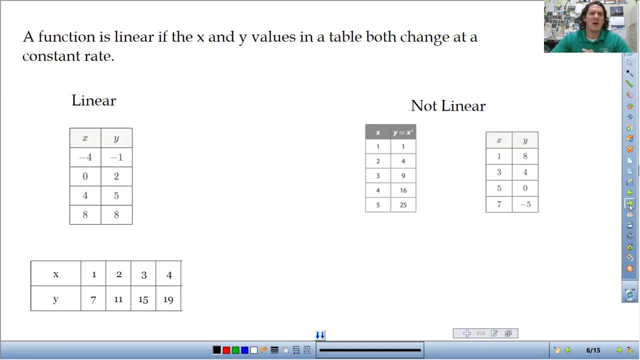 be looking at the points in the table. So a function is linear if the x and y values in a table both change at a constant rate. So couple of examples here of linear and not linear. So here this is linear. So if you, 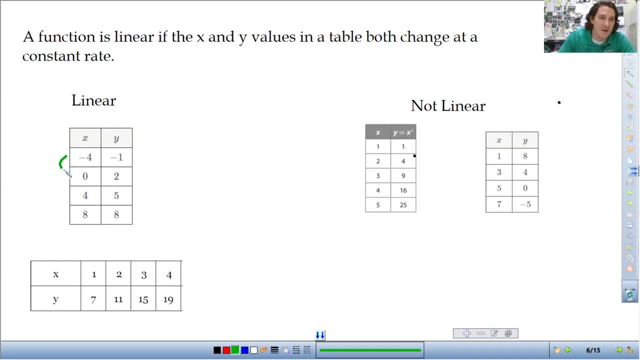 look at the x values. The x values are increasing by four each time. All right, the pattern is to increase by four. Then, if you look at the y values, the pattern is increasing by three, And so the x values are increasing. 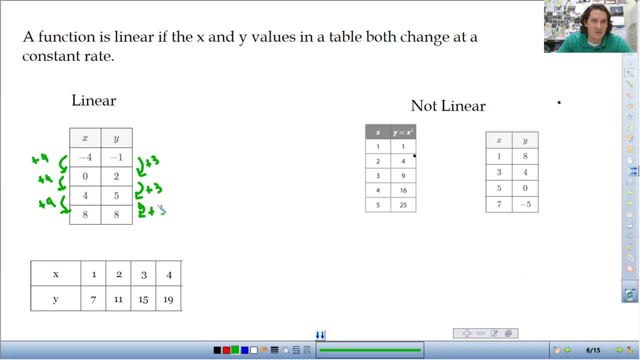 by a constant rate and the Y values are increasing at a constant rate. that makes it linear. so here on this one, the X values are increasing by 1 each time. so plus 1 plus 1 plus 1, you can do a different color for the Y values. the Y. 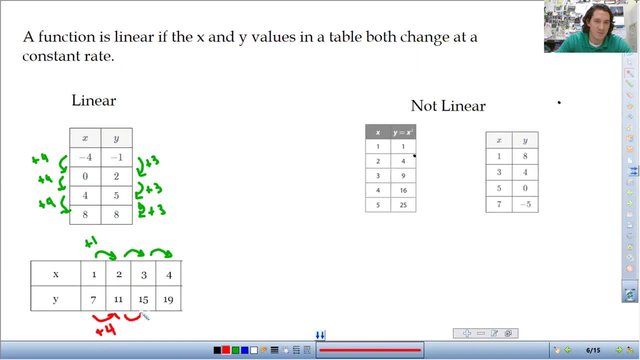 values are increasing by 4 each time. so plus 4, plus 4, plus 4. that makes it linear. so here we look over at this. the X values increase by 1 each time, so plus 1, plus 1, plus 1. but then look at the. 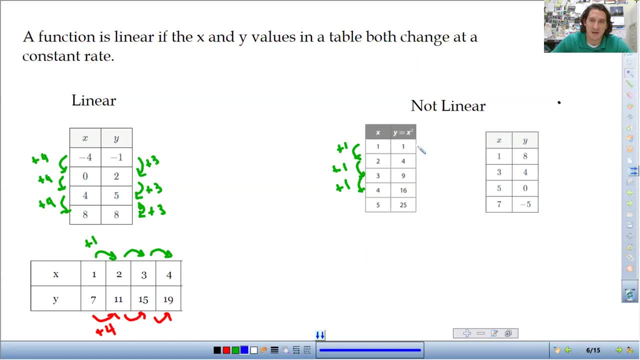 Y values. they are not increasing at a constant rate. so Y is plus 3 here, but then it goes to plus 5 and then it's it's plus Seven. so there is a pattern of how it increases, but the numbers need to be the same. 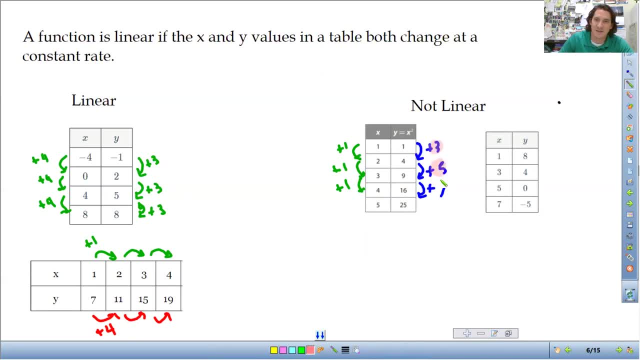 So this is the issue here. These are not the same, so not linear. One more example of linear and not linear, or, excuse me, not linear. here. These increase at the same each time: It's plus one, plus one, or, excuse me, It's not plus one, It's plus two. 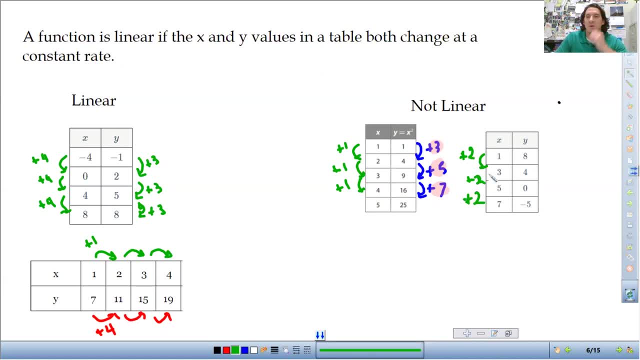 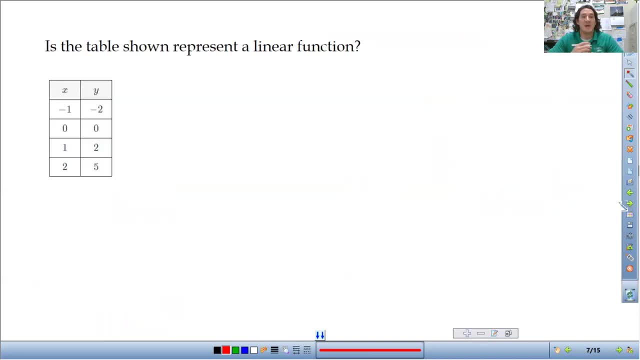 These are not, so not linear. So let's look at a few examples. is the table shown? a Represent a linear function. a So negative one, so negative one, Zero one, two. So the pattern here: they all increase by one. so plus one, plus one, plus one. 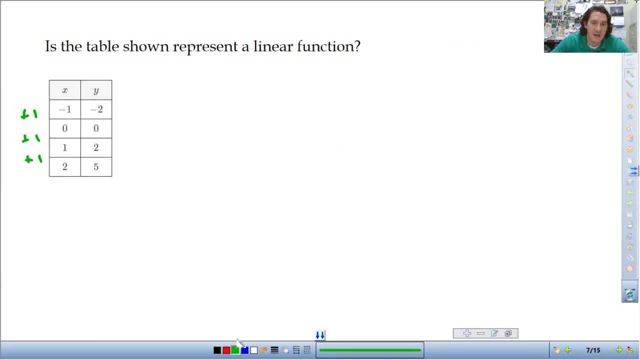 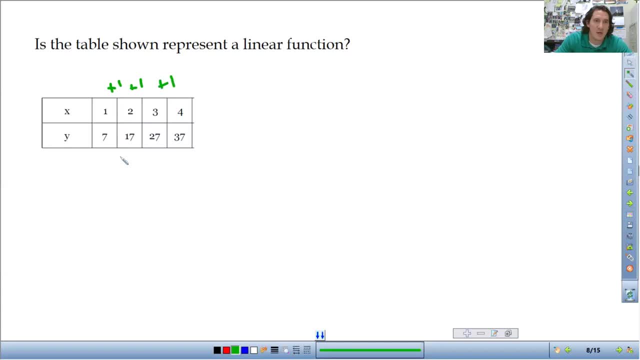 increases plus 1 plus 1 plus 1. down on the bottom, The y values is plus 10 plus 10 plus 10, both increasing by the same amount each time. So this is linear. This is a linear function. And then you could also speak to: theünüz is a linear function. 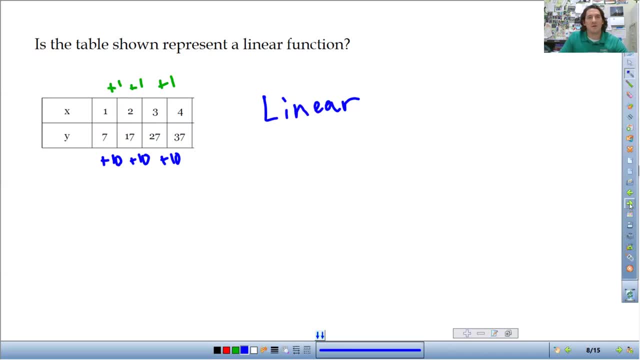 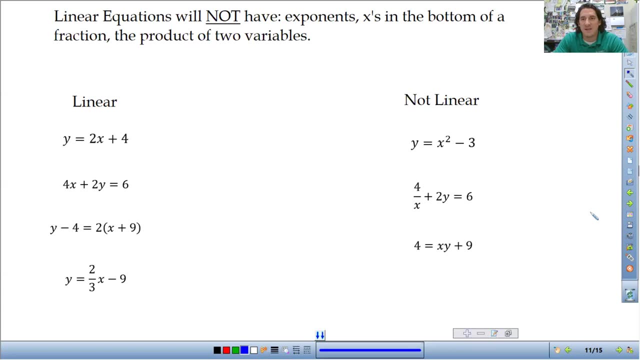 All right, we're gonna skip ahead a little bit. So linear equations. so if you're just looking at the linear equations, they will not have these things. exponents in the bottom. exponents: x is in the bottom of a fraction. 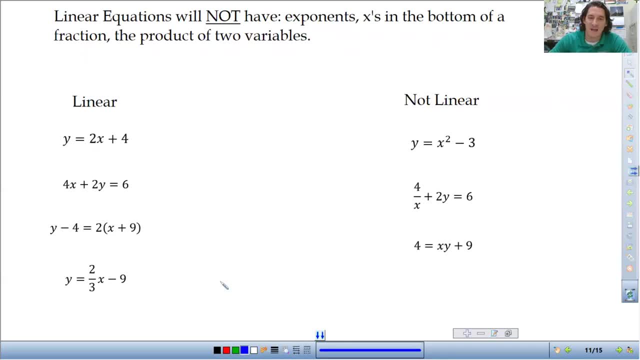 or the product of two variables. Let's actually talk about the non-linear stuff first. First one: this one's not linear because here as an exponent, so not linear. This one: here the x is in the bottom, So not linear. 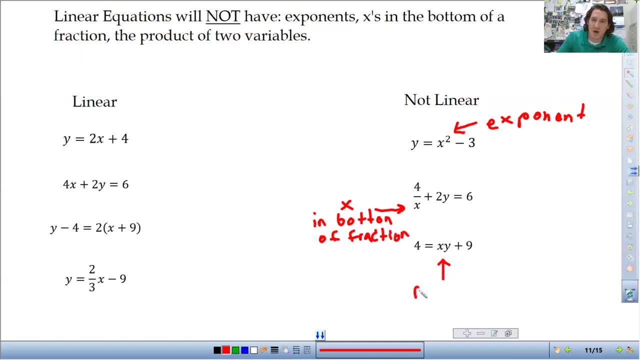 And then this last one. this is the problem. this is the product of two variables. So when we see these things again, exponents x is in the bottom, or the product of two variables. that tells us it's not linear. So all. 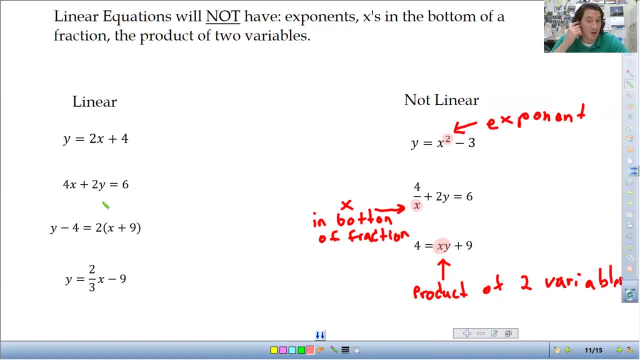 these over here are linear. These are actually the most common examples of linear functions that we are going to be dealing with a lot this school year. These are three common. this is called slope-intercept form. this one is standard form. this is point-slope form. 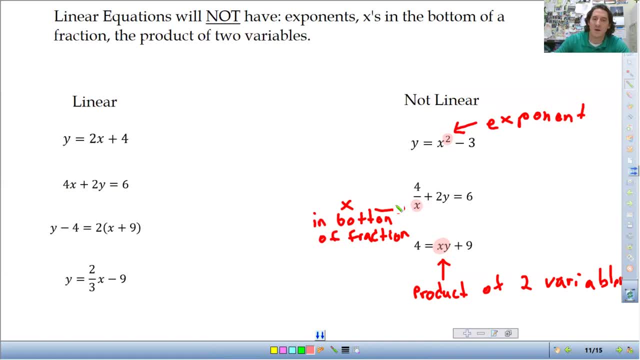 These are all linear. One thing I want to point out is that this is not linear. One thing I want to point out: a linear function can have fractions, So this has a fraction. this is fine. the x is not in the bottom of the fraction. 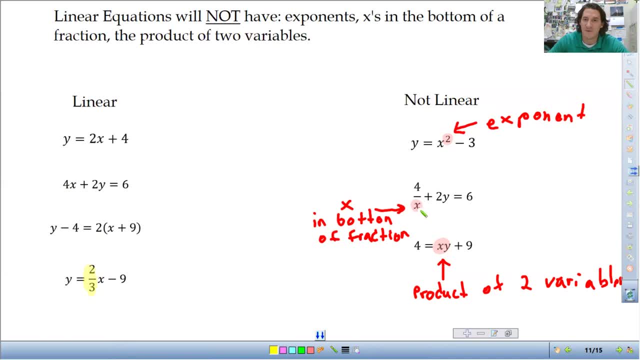 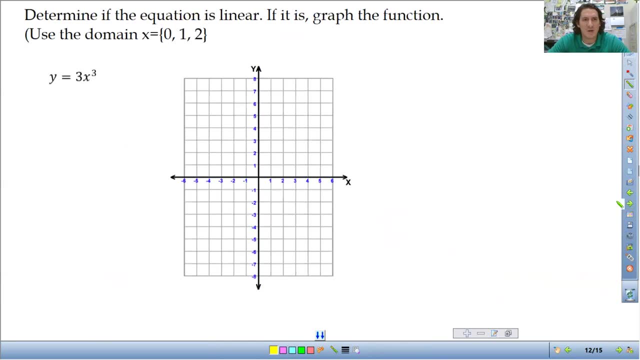 That's when it can't be linear. So fractions are okay, but if there's an x in the bottom of it, not okay. So these are all linear. So let's look at an example: Determine if the equation is linear, If it is graph the function, If we're going to graph it, we're going to use the. domain. just to keep it simple Right off the bat, if this is the curve, it's going to be a 1,, 2,, 3,, 4,, 5,, 6,, 6,, 7,, 8,, 7,, 9,, 10,, 10,, 10, and 12.. 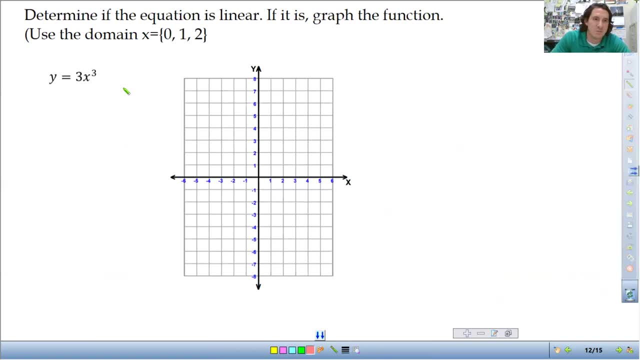 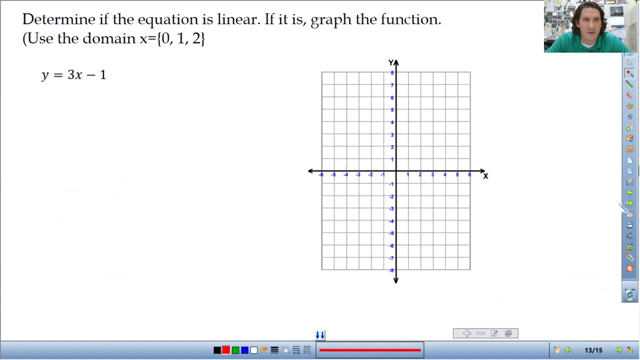 If you do this, you're going to get an equation which is going to have an So right off the bat exponent. Since it has an exponent not linear, we don't need to graph it All right. Next one: determine if the equation is linear. 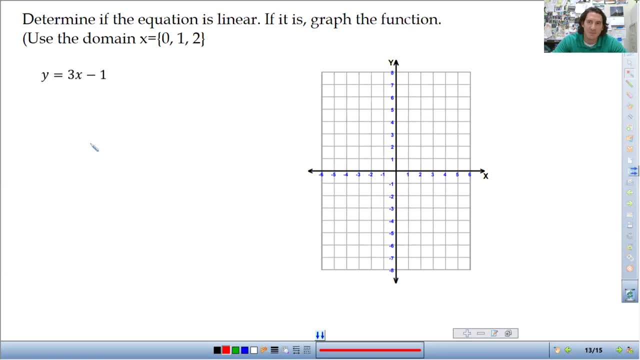 If it is graph the function. So, are there any exponents? No, Is there an X in the bottom of a fraction? No. Is there a product of two variables, like an X times Y? No, So, yes, this is linear. 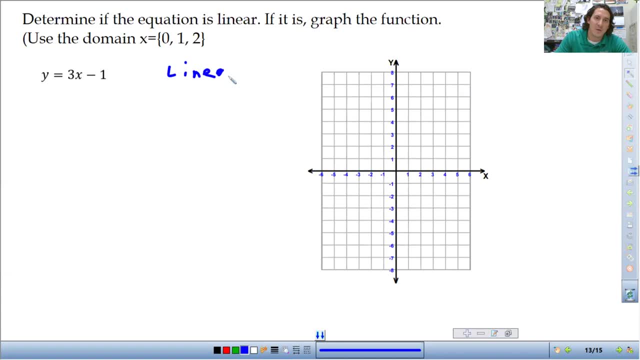 All right, And so we are going to graph it using this domain, just like we did in the last unit when we were graphing functions. So I'm going to take my X value, starting off with X equals zero. The function is: Y is equal to three times X minus one. 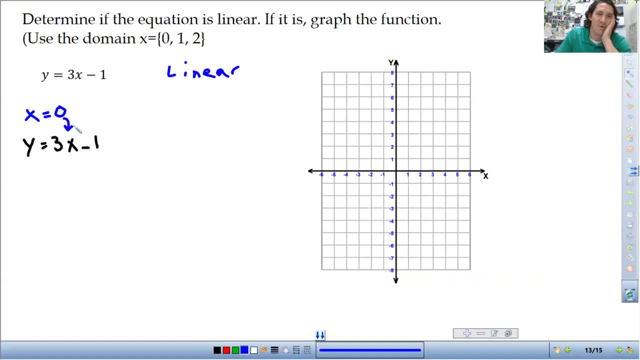 And the zero is going to go in for X, So it's going to be three. So three times X, and again X is zero. So three times zero is zero minus one is negative one. So from there I get the point: zero negative one. 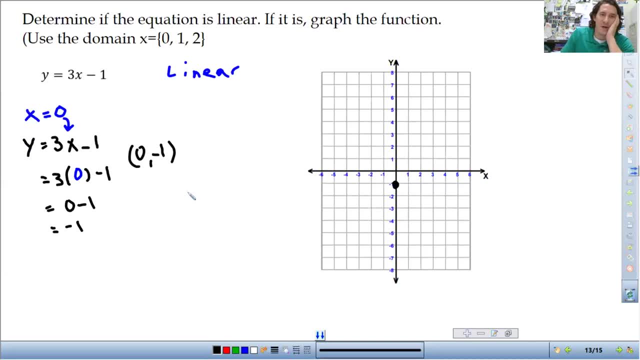 I'm going to plot the point Zero negative one. I do the same thing for X equals one, So with the function Y is equal to. So Y is equal to three times X minus one. I'm going to put the one in for the X. 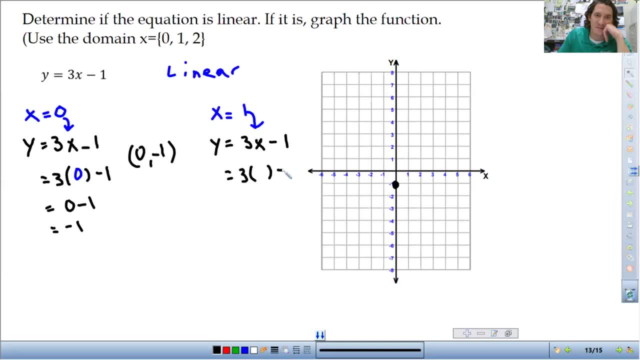 So it's going to be three times X minus one and X for this one is one. Three times one is three minus one is two. So I'm going to plot the point: One, Two. So that's one on the X, two on the Y. 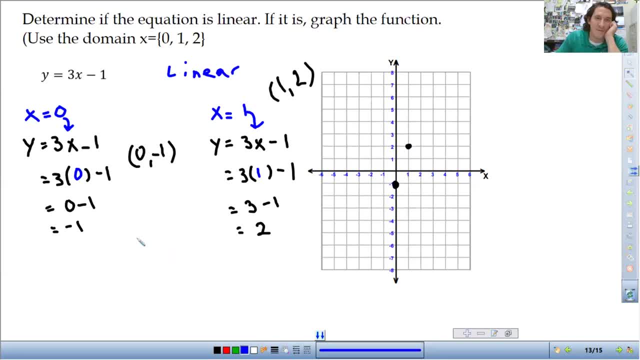 Put a point And then I need to do that one last time. for X equals two, So it's going to be: Y is equal to three times X minus one, and the two is going in for X. So three times two is six minus one. 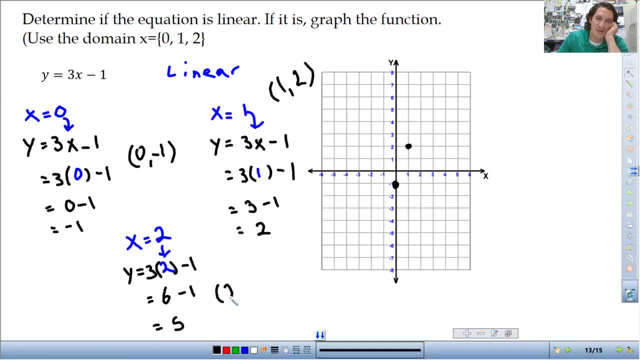 Six minus one is five, So I get X is two, Y is five. So two on the X, five on the Y. Put a point. We're just plotting the points, so that's all we need to do. Notice that all three points line up in a straight line. 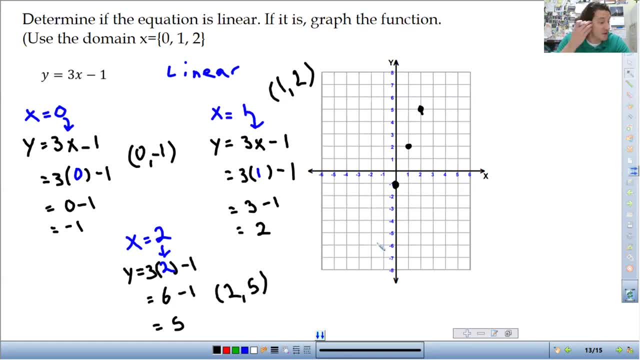 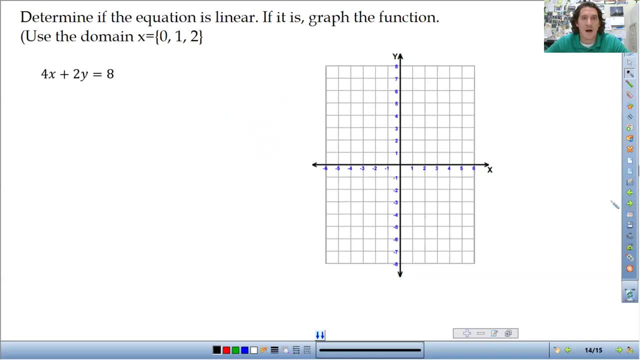 You don't need to connect them with a line yet. We're not at that point yet. We are going to do that eventually with these graphs. But right now, just plot the points, All right, Determine if the equation is linear, If it is graph, the function. 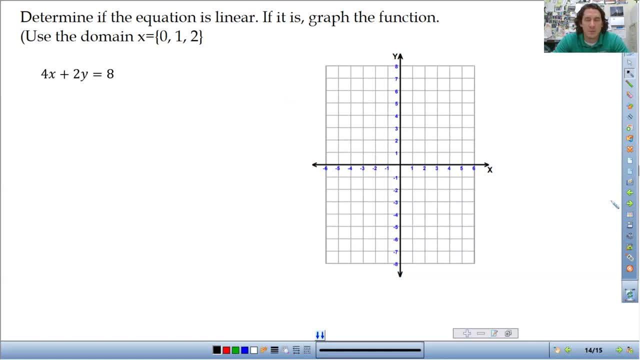 So we're going to use the domain 0,, 1, 2 if it is a linear function. So again, what we want to look for. Are there exponents? No, Are there X's in the bottom of a fraction? 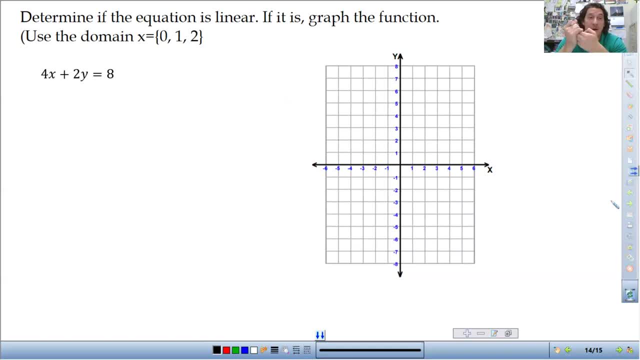 No. Are there any products of two variables, So an X times Y? No, So this is linear, So we have to graph it. So this is going to be a little bit different for graphing it, because it's not. 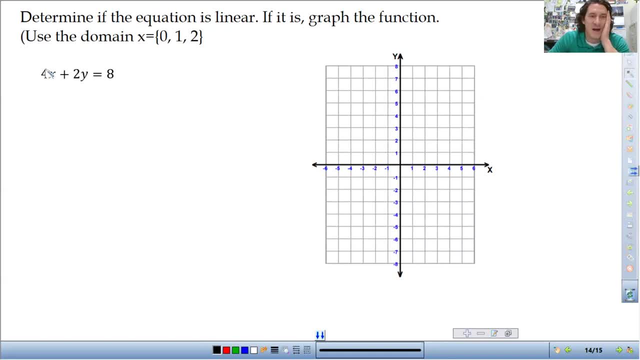 We can just use a table and put in the X value, the 0,, 1,, 2, and the X and then solve for Y. That's fine What I'm going to do, so we don't have to keep solving for Y over and over again each time we work this out. 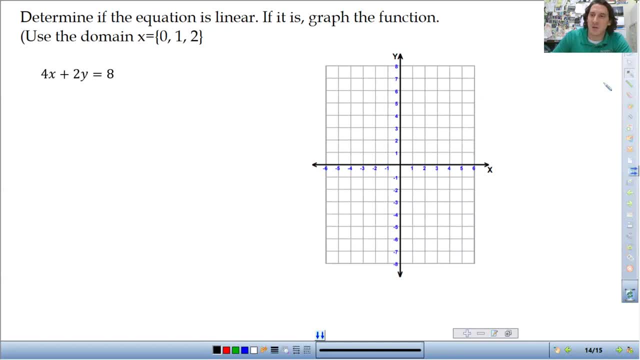 I'm going to solve for Y first. All right, Just like what we did yesterday or in the last lesson, I'm going to get Y by itself, on the left side of the equation. So first thing I'm going to do is eliminate the. 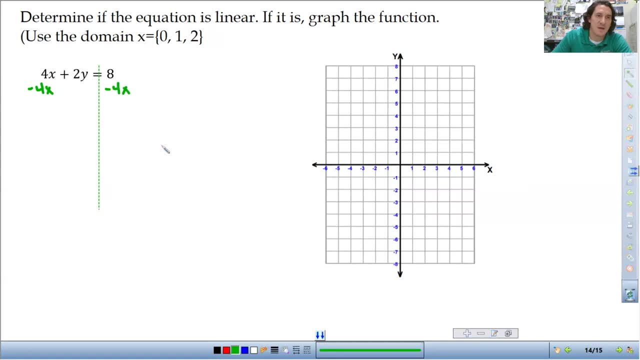 4X from that side. So I'm going to subtract 4X. So positive 4X minus 4X cancels out I get. 2Y is equal to 8 minus 4X. You can write as 8 minus 4X. 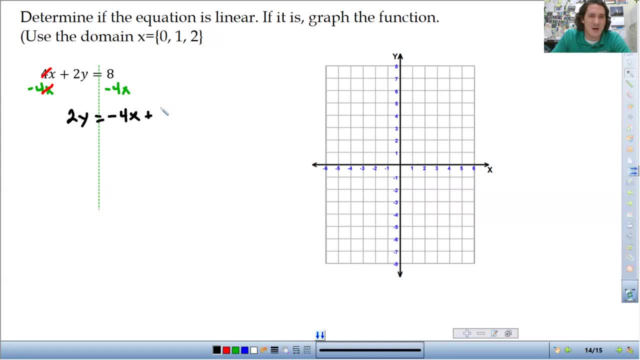 We need to get used to seeing that as negative. 4X plus 8.. So that's how I'm going to write it, And then I'm going to eliminate the 2 by dividing everything by 2.. Divide everything So the 2s cancel out, and cross that out in red. 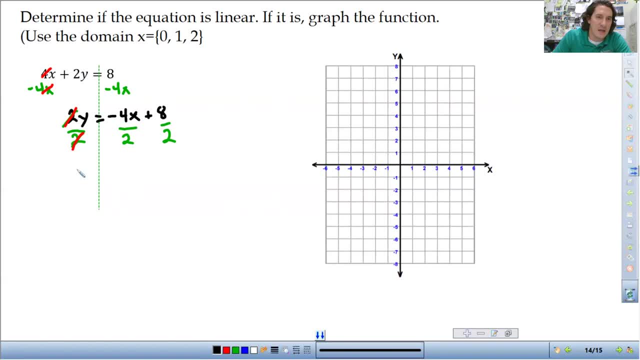 So the 2s cancel out and I get: Y is equal to negative. 4 divided by 2 is negative. 2 plus 8 divided by 2 is 4.. So here is the function that I'm going to graph. 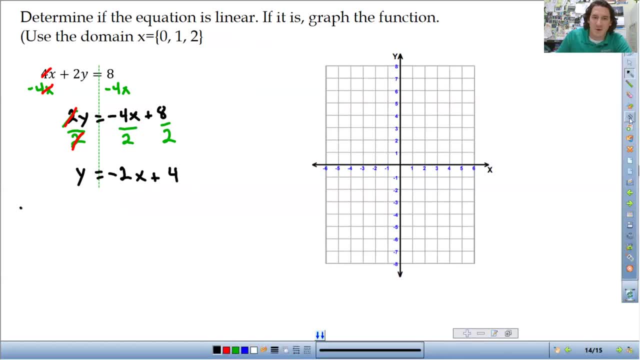 And I'm going to streamline my work a little bit. I'm going to use a table this time. You can do either method. You can just put your work wherever you want, Or you can use a table, Like what I'm about to do. 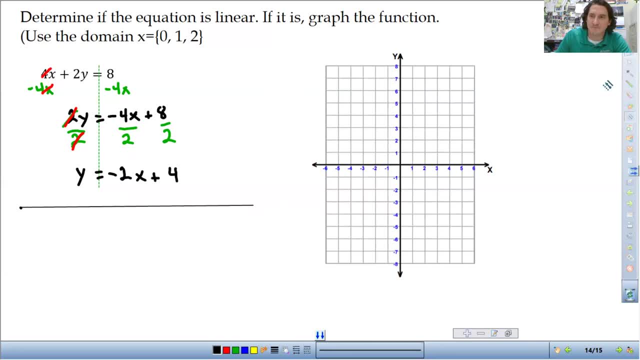 Either way is fine. You're doing the same thing each time. So use the domain 0,, 1,, 2.. So first it's going to be using the function, So it's going to be negative 2 times X plus 4.. 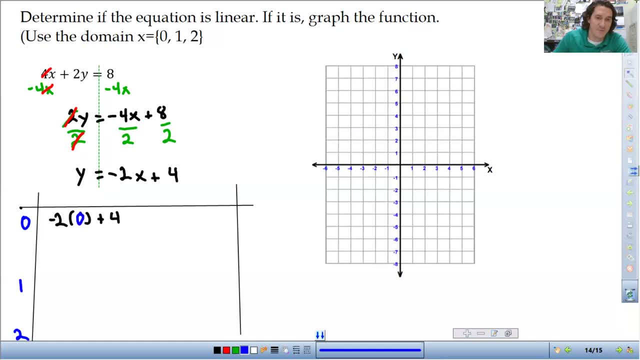 Negative 2 times X Or X. So negative 2 times X is 0 for this one. Negative 2 times 0 is 0 plus 4 is 4.. I'm going to move this over a little bit, So I don't need that much space. 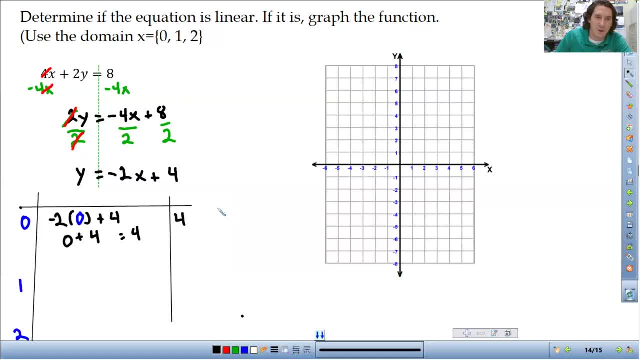 So when X is 2, Y is 4.. So I'm going to plot the point: X is 0, Y is 4.. So 0 on the X. I don't move left or right, I go up 4.. 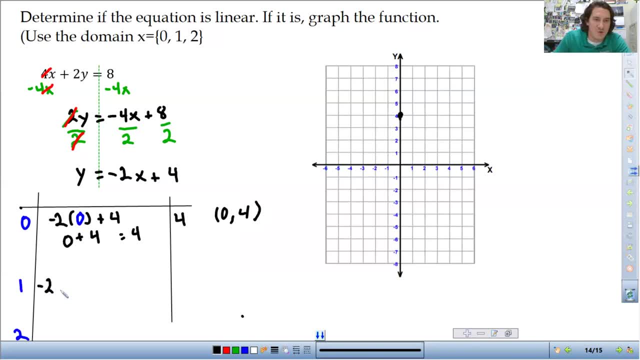 Put a point, All right. Next I'm going to do negative 2 times 1 plus 4.. Negative 2 times 1 is negative. 2 plus 4 is positive 2.. So I'm going to plot the point 1, 2..